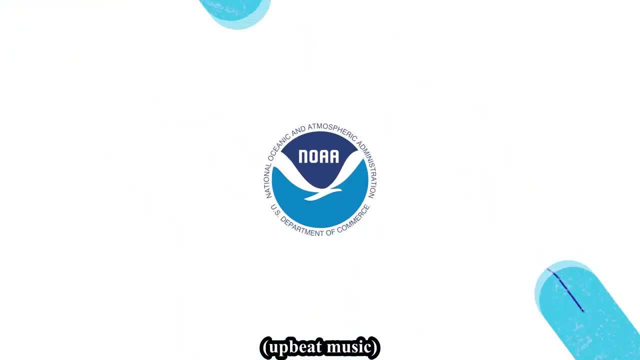 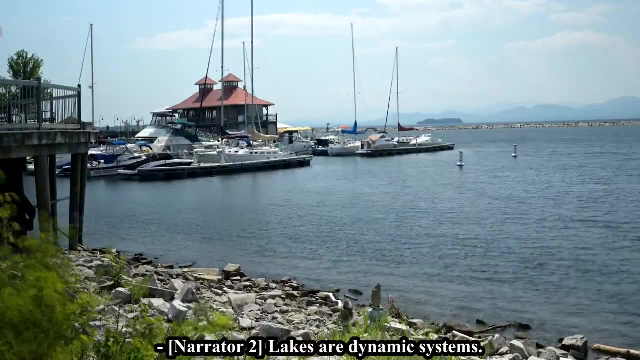 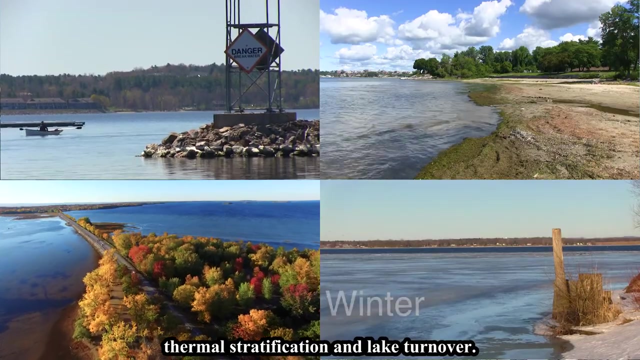 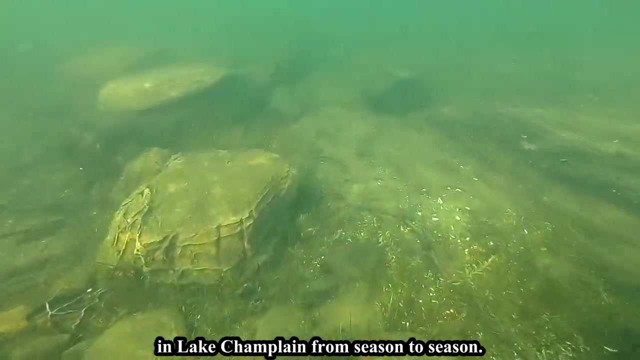 the Lake Champlain Basin. Lakes are dynamic systems. Throughout the year, Lake Champlain experiences thermal stratification and lake turnover. What happens is occurring below the surface of the water in Lake Champlain from season to season? First, what is lake turnover? 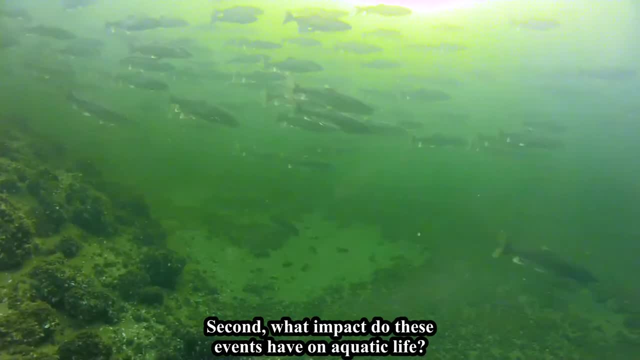 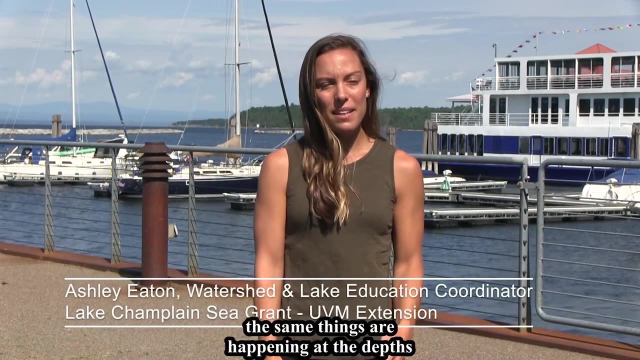 Lake turnover and thermal stratification. Second, what impact do these events have on aquatic life? In the same way we visualize shifts in the landscape, the same things are happening at the depths of Lake Champlain throughout the course of the year, with the changing of. 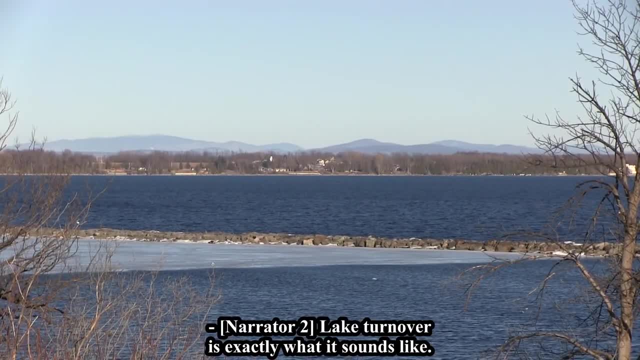 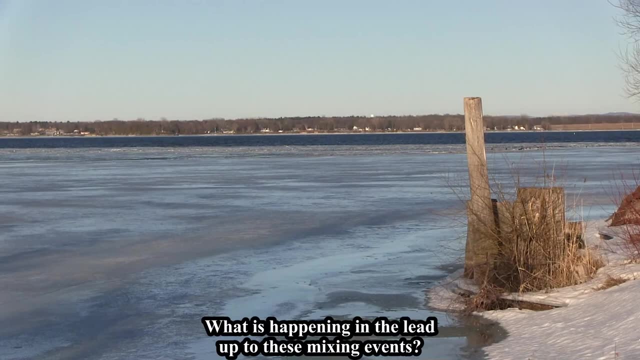 the seasons. Lake turnover is exactly what it sounds like. Water moves from the top of the water column to the bottom in a mixing event. What is happening in the lead-up to these mixing events? Thermal stratification is the process in which the lake becomes divided into layers. 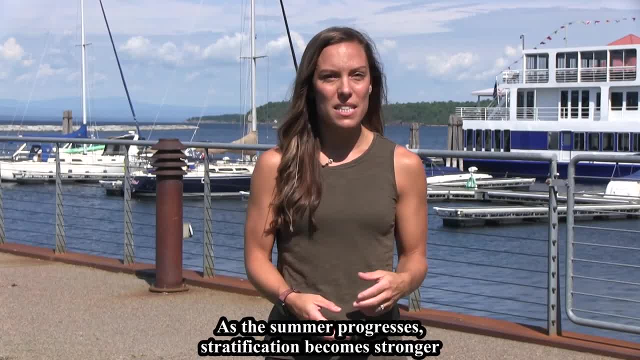 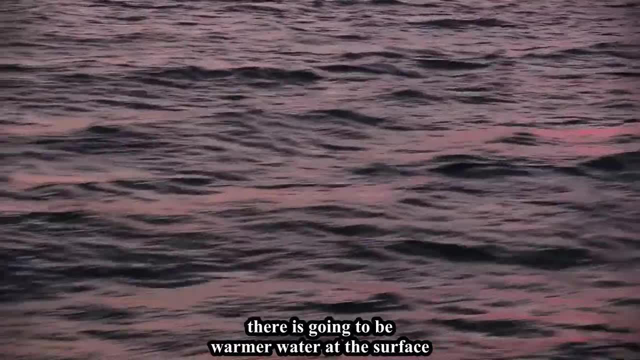 based on water temperature and density. As the summer progresses, stratification becomes stronger and will create niche segments throughout the water column. When the lake is stratified, there is going to be warmer water at the surface and colder water at the bottom of the lake. 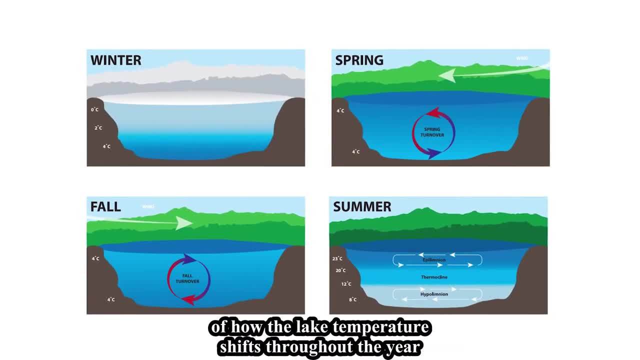 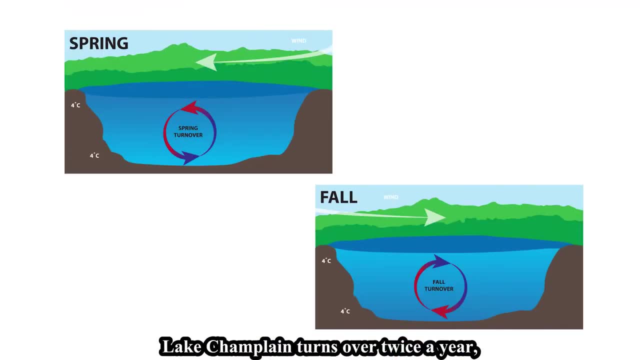 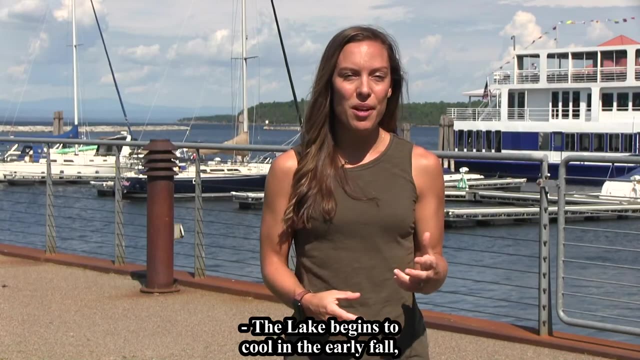 What you are seeing right now is a visualization of how the lake temperature shifts throughout the year, based on physical effects in the atmosphere above. like temperature changes and winds, Lake Champlain turns over twice a year, Once in the spring and once in the. The lake begins to cool in the early fall, taking cues from decreasing air temperatures. 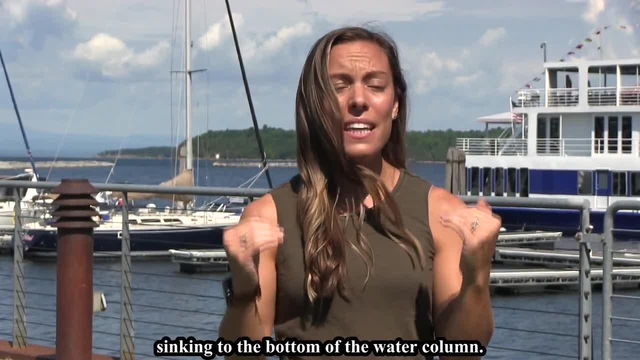 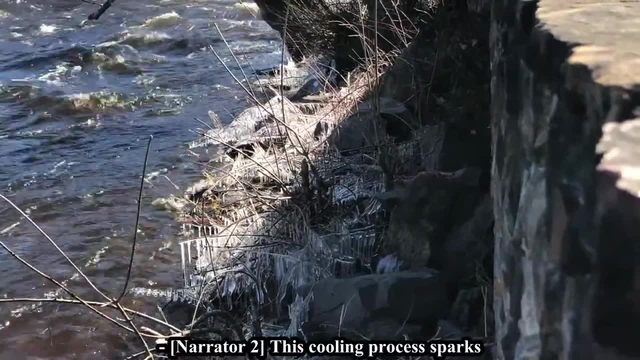 This cooling process shifts the density of the water and denser water is heavier, sinking to the bottom of the water column. When it does this, it actually forces the warmer water to the surface. This cooling process sparks one of the annual lake turnover events in Lake Champlain. 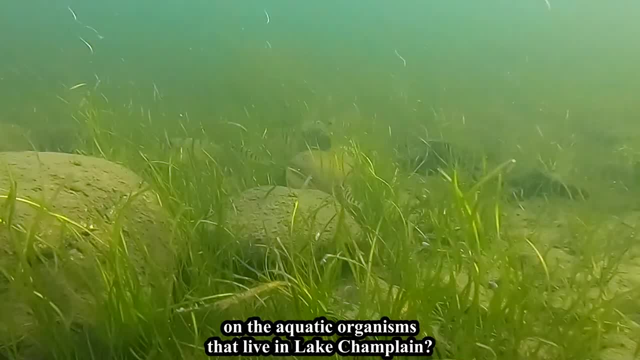 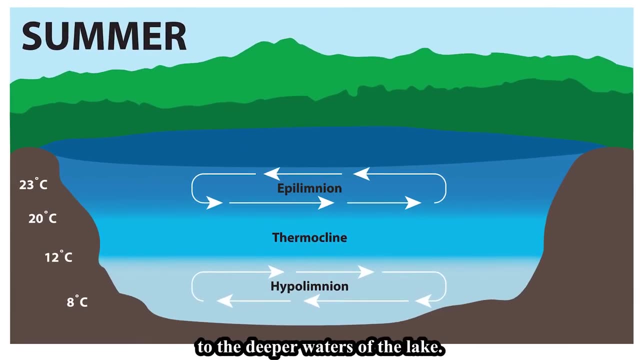 What impact does this have on the aquatic organisms that live in Lake Champlain? Lake turnover is an important phenomenon because it allows for the redistribution of oxygen and nutrient-rich surface waters to the deeper waters of the lake. In the fall, wind moves highly oxygenated surface water to the bottom of the water column.